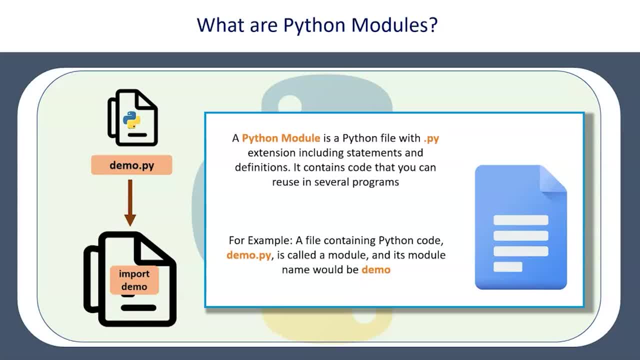 few set of administrators or the senior developers can maintain and pass it on to the team. Now, for example, a file containing Python code- demo dot py file is- will be called as a module and its module name would be demo. So you need to take care that, whatever the name of the file is, 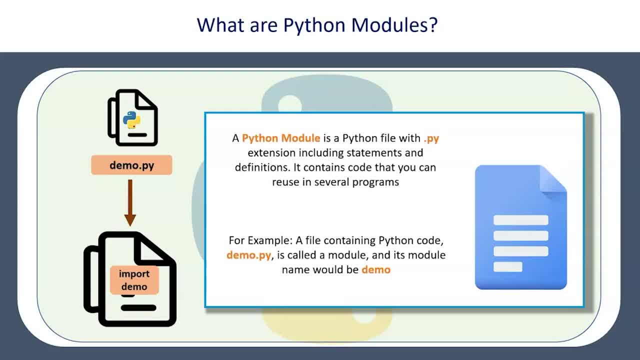 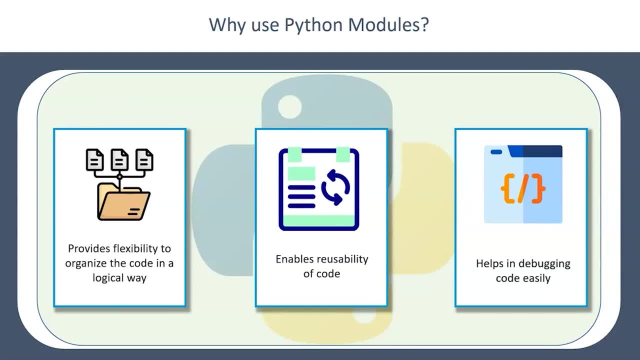 that is what will get imported in your Python code. So we will see that with our certain examples on our Jupyter notebook. Now, what do we need to use? As I have reiterated, it provides flexibility to organize the code in a logical way and it enables reusability. 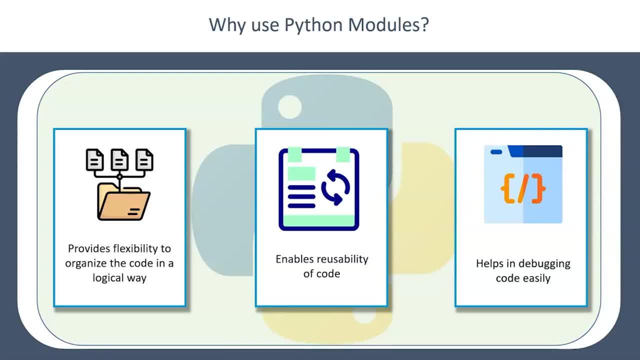 which is the most important factor. So one: of course you can organize the code. you keep the reusable code at one place or you can keep a modular approach and also reusable. So no, not all the developers have to go and rewrite that code, And it is easy to maintain and helps in. 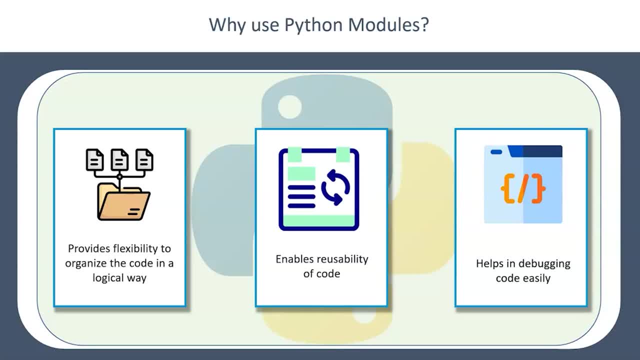 debugging the code easily. So if you know that there is an error coming, there is an issue coming in one of the modules which is imported or which is lying in the common file, then it becomes easy to debug. You just have to go and check that particular function. You don't need to go and 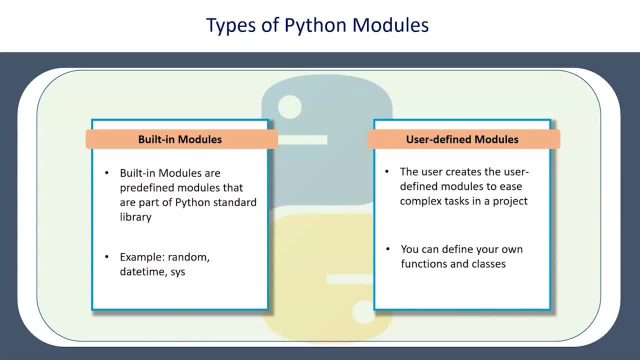 check in each and every piece of code. Now, there are two types of Python modules. Definitely, there are built in modules which Python library provides, which you don't need to import explicitly, But there are certain user defined modules which you can use to do that. So, for example, if you want to use Python modules, you can use Python. 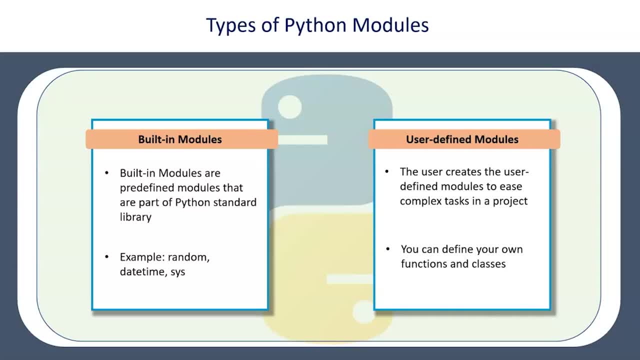 modules which you create on yourself for your own custom development, for your own custom programming. So built in modules are predefined modules and are part of the Python standard library, for example random date time sys. So we will take a look at these examples also. 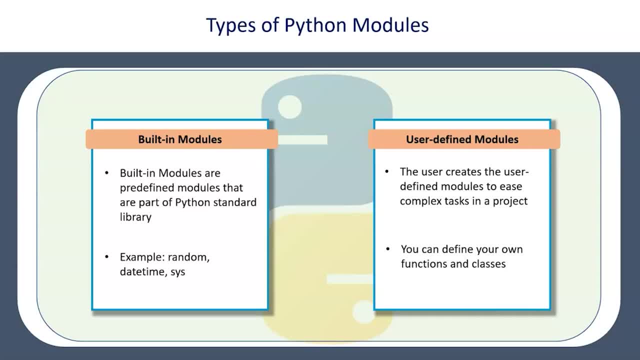 And, of course, the user defined modules, which is the primary objective of this session, where we're going to show you how do you create your own defined modules and then import them. So the user creates the user defined modules to ease complex tasks in a project. So you program the complex piece of the code in a common module. 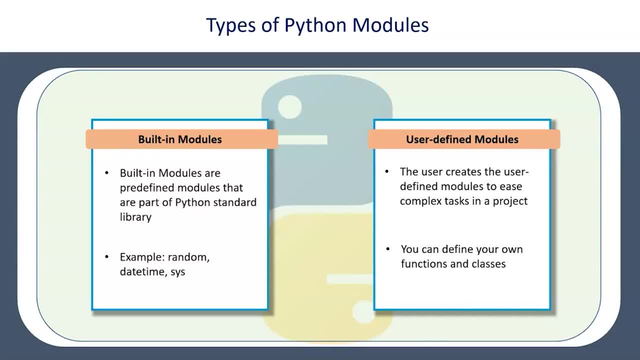 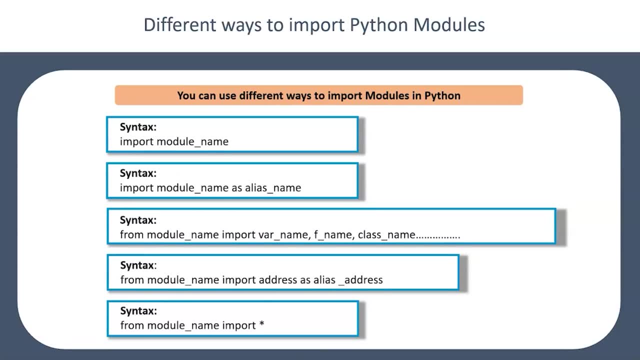 and give it to everyone. You can define your own functions and classes. Now, what are the different ways? There are five different ways. you can import modules. So you can just say import module name and all the classes and functions within that module will get imported. You can give an alias. So basically, you can give an alias to the module. 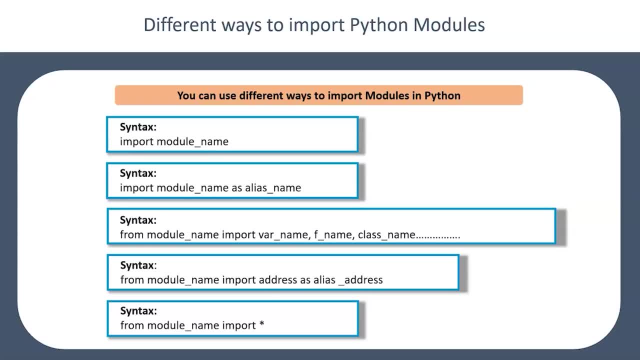 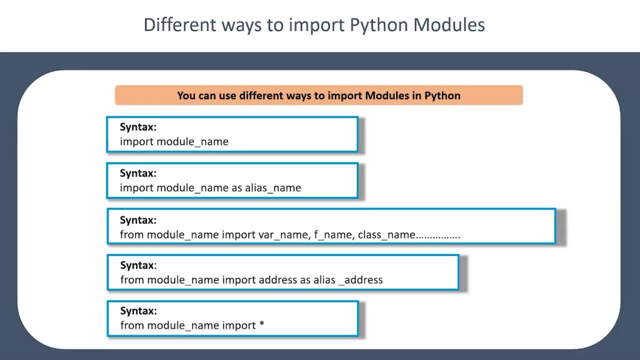 Then if you want to import anything specific from the entire module- you don't want to import all the functions and classes- then you can just import the specific functions and classes and give their name. Then fourth is from module. you want to import any address as an alias? You can import and give an alias to the specific. 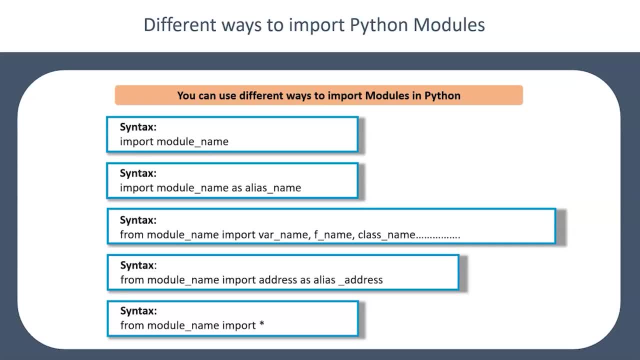 the class name and then, of course, similar to the first syntax, you can module all everything. so first and the last syntax are almost having the same meaning: to import everything in your module. okay, so with this background, let's first take a look at the Python file. so we have what we have. 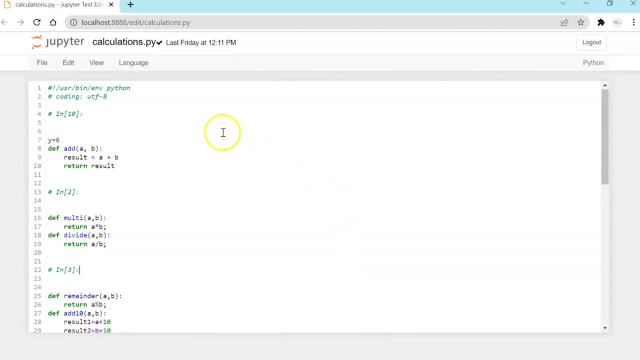 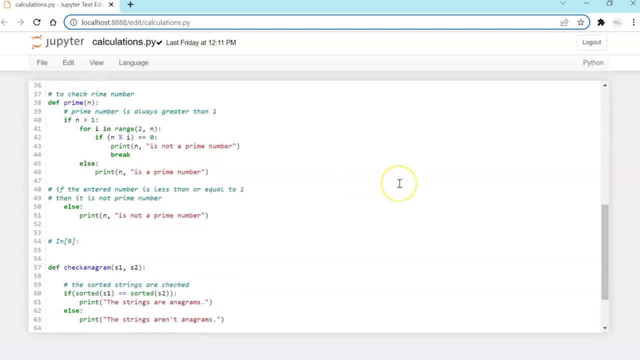 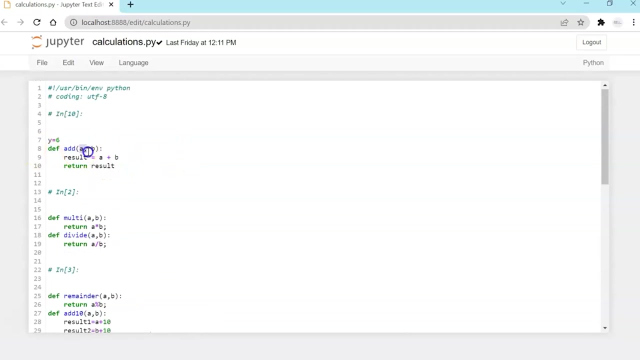 done is we have created a module, calculations, dot py. so just please focus on the part where the name of the file is calculations. and in this Python file, dot py file, we have created a couple of functions and the relevant logic related to those functions. so very simple functions like addition, add, you pass two. 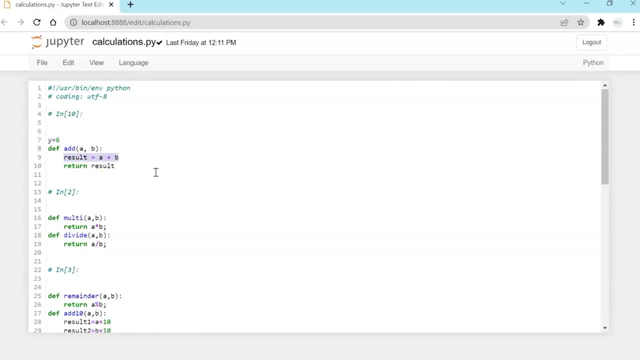 variables and you send the result. add the variables and send it back. basically, we are overriding the Python internal operator add in our Python module and we will be invoking this one. so will show you how to invoke. then you will have. I have written multiplication division remainder. so you two, you passed two variables, divide them. 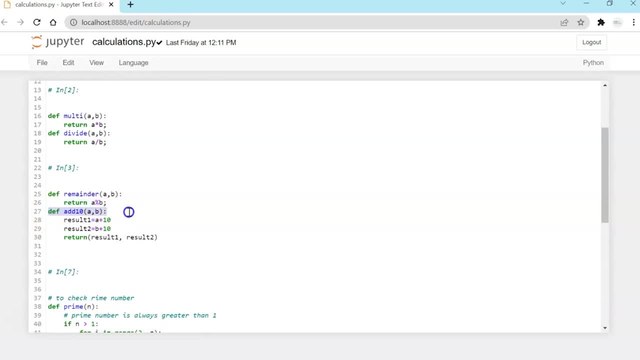 and find the remainder. then now a custom function where I am adding ten to both the variables which are being passed to this function and returning the result. then there is a function which checks whether the number is a prime and if it is not a prime number you will get. 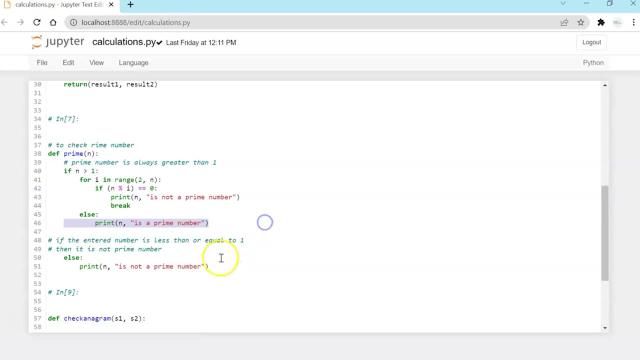 get this output and if it is, you will get a is a prime number, okay, and then another function which says check anagram. so we will just sort the two strings which we will send and check both are equal or not. if both are equal, then the strings are anagrams, otherwise they are not. so these are. 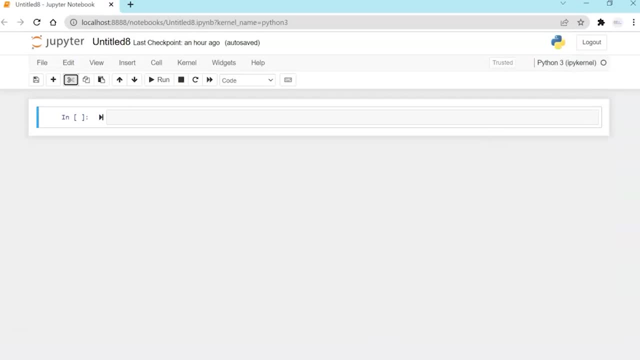 the set of functions which you have written. now we will see how will we use them in our code. now, first syntax which I am writing is import calculations. so this is the name of my dot py file, which is residing in the same folder where I am writing this piece of code. and now, if you 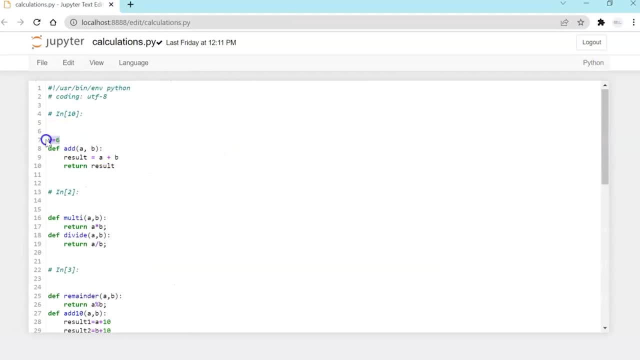 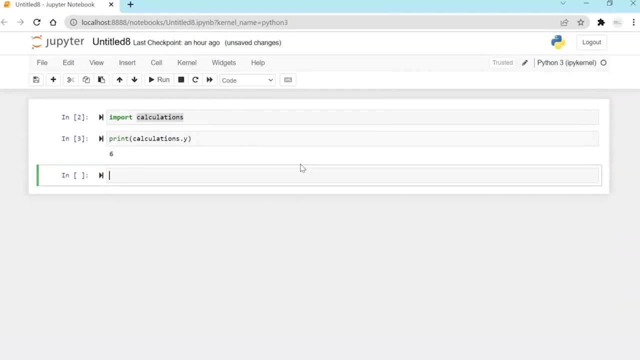 see, in my dot py I have a variable- why- whose value is 6. so I'm just using that value and running it and printing it. I'm just going to show you how expensive it is to use that value explicitly. I'm invoking the functions in the calculations class in the calculations dot P. 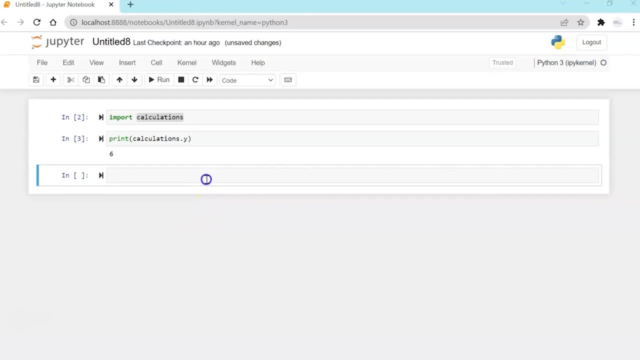 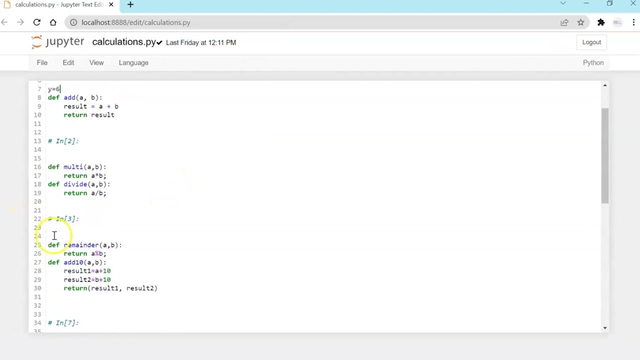 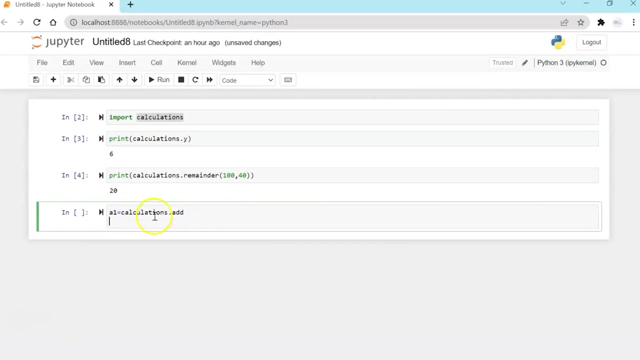 by 5. okay, now let's invoke another function remainder, passing 140, and then I should get 20 as an output. okay, so this has gone back and executed this particular function. now what I'm going to do is another example of my addition. I'm saying calculations, dot add. I'm going to initialize and. 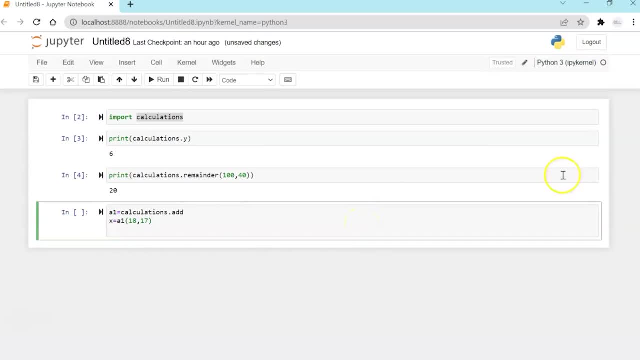 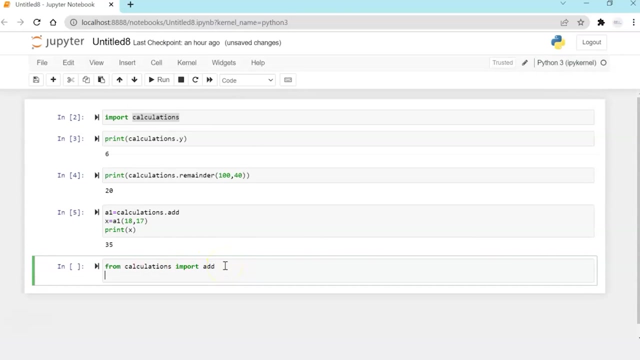 pass two variables and my expected output is 35. okay, so it has gone and executed this function. now I'm going to show you another syntax of importing. so from calculations. I'm just importing the add action. length row is very simple, so on this side we do not need to do that. you need the add function. 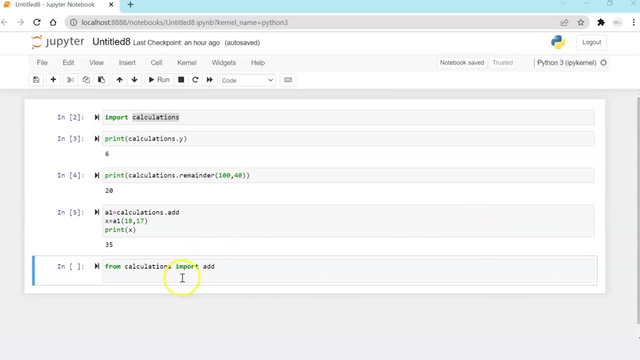 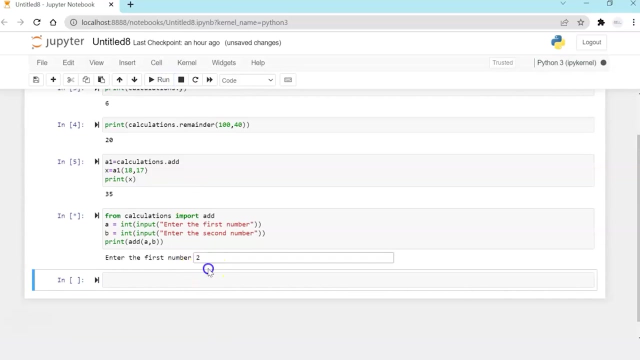 function. so I'll ask for user input to enter for one and two numbers, and then I'm just going to add it two and five, so I got my output is seven. now the difference to be noted over here is that in the previous syntax I was making a. 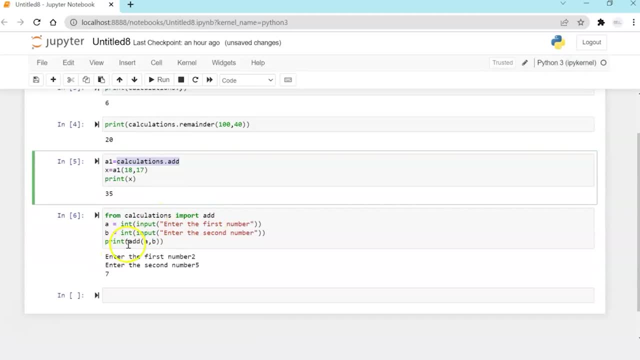 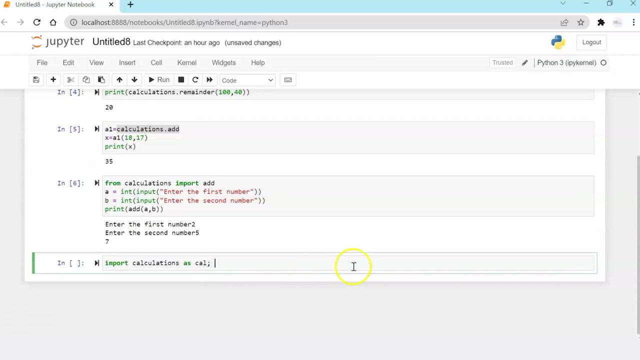 call like calculations dot add. but now I don't need to make a calculations dot add syntax invocation, I just need to say import add and I just need to use the add function. that's all. now let's use another syntax to import modules. so I'm using import calculations as cal, so all the modules are imported but the alias. 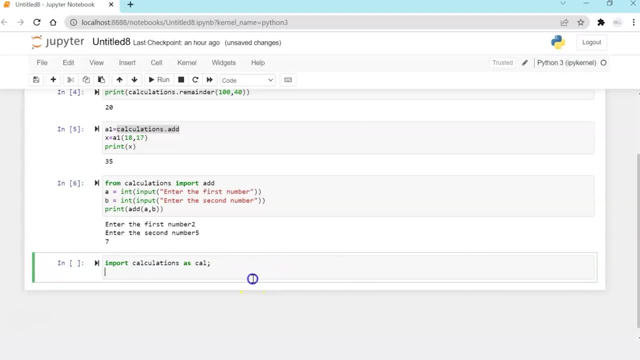 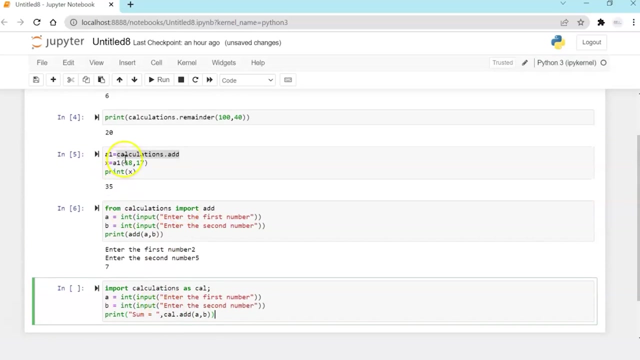 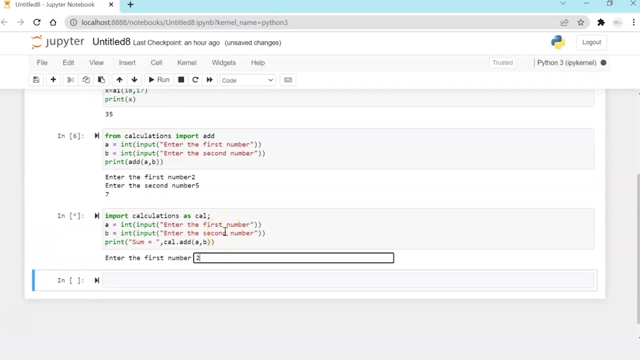 uses cal and similarly, like the previous example, I'm going to take two inputs and print the sum. now, the difference in this syntax? in this syntax is I'm using the alias cal dot add, but my output should be seen you, okay. similarly, I can call prime, whether it's not a prime or prime number, I can. 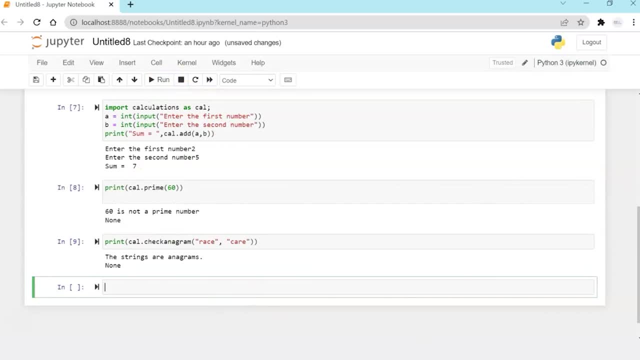 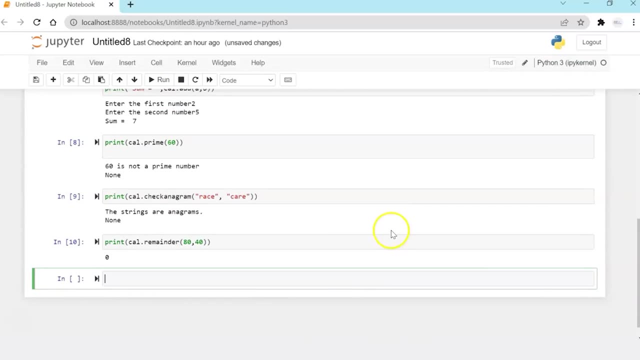 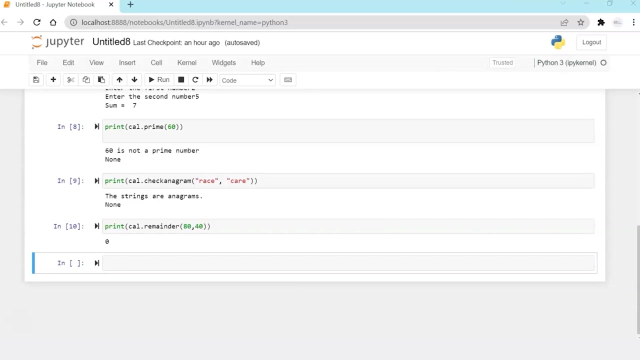 call the check anagram using the same alias and I can call the remainder function, okay. so I hope you have noticed that the difference in importing, the way of importing the module, makes a lot of difference. right now let's take another example of importing some functions or variables. so 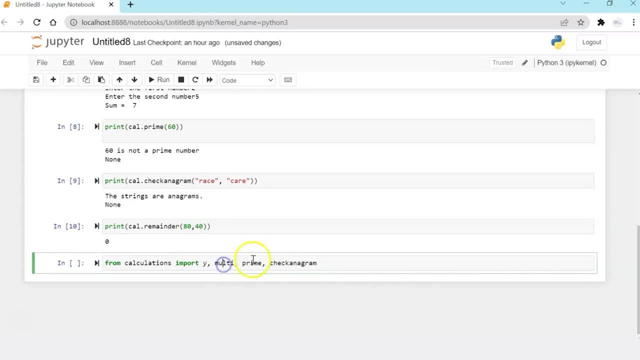 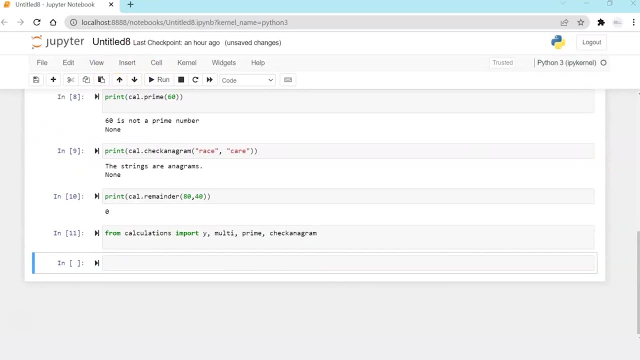 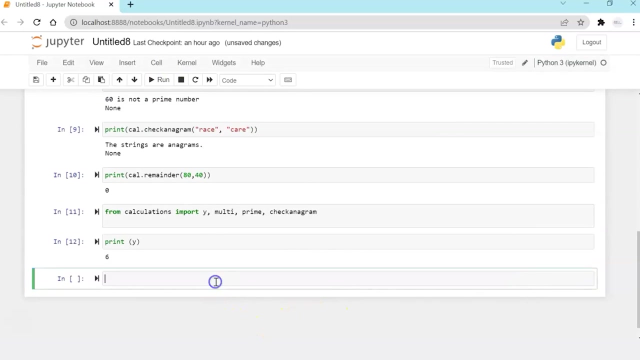 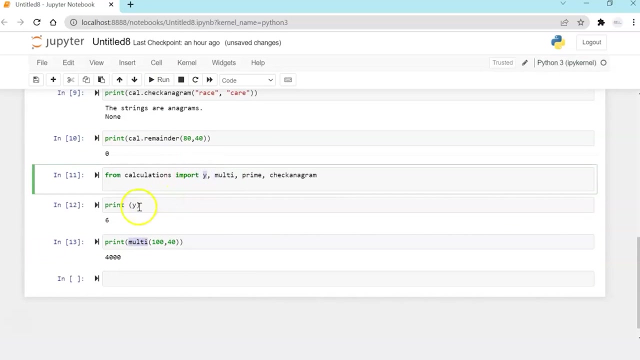 I'm going to explicitly, I'm importing my variable Y and functions multi, prime and check anagram explicitly and I'm going to print Y, okay, and I'm going to multiply two numbers. so if you see, I'm using these aliases over here, okay, I'm using these variables. 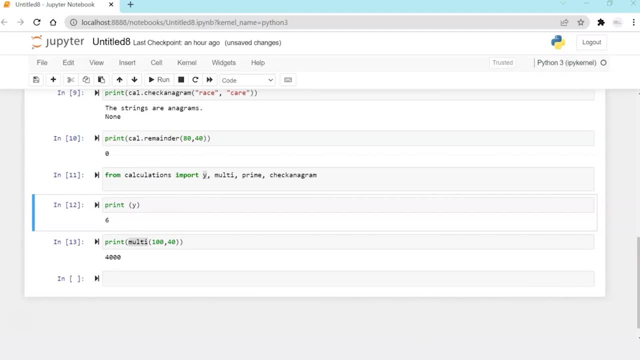 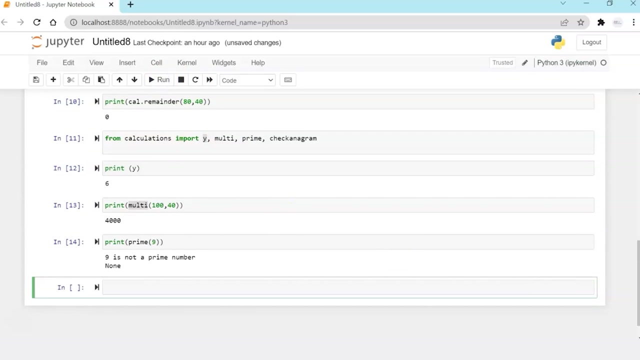 directly, as I've already imported. now I'm going to say prime 9. now it's printing none. if you see, it's because of the statements which are not executed right. so that's the error there. so that's profahrt right. so that's why you are seeing. now let's check anagram. 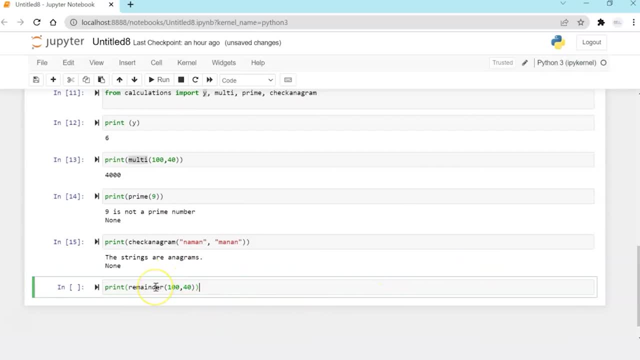 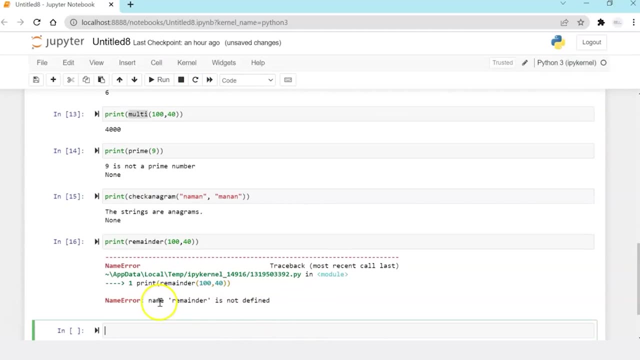 and now, another thing to be noted is i'm trying to invoke a function remainder which i have not imported over here. so let's see how what error python throws. okay, so yeah, so python has throws an error that name remind remainder is not defined because i have not imported it over. 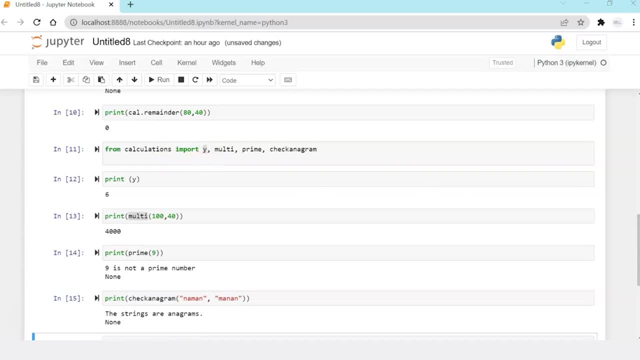 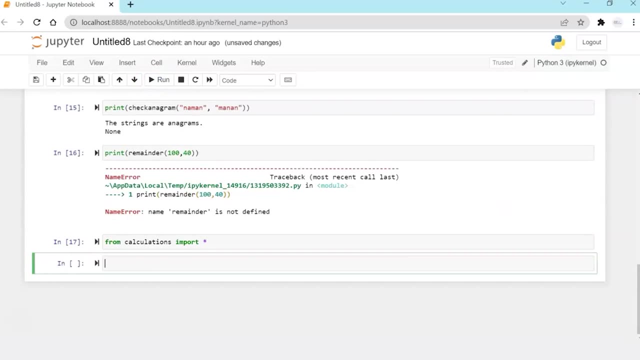 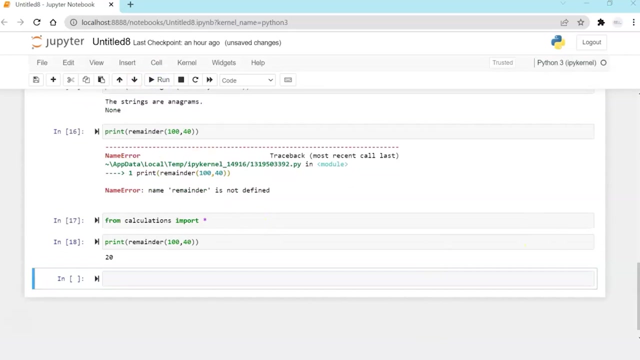 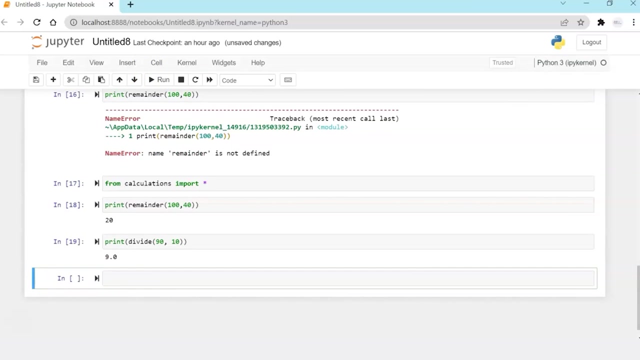 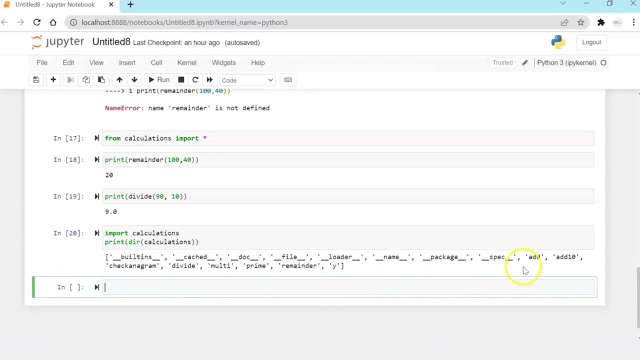 here. so now, in order to import remainder, what i am now doing different is importing all the functions. now, if i use remainder, it should run. okay, i am using divide, okay, cool. now i am going to show you another function, which is a utility function, directory function, which will show me all the functions, variables, as part of the python file. 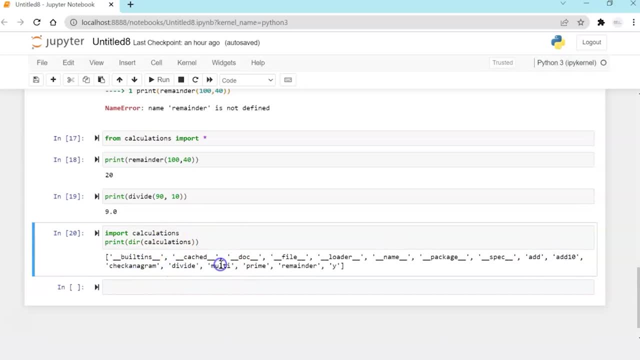 add, add 10, check anagram, divide, multi, prime, remainder y. and of course, these are some inbuilt packages, uh, which are already there in the python file as part of the python loader, but these are the ones which i have created so you can actually see the list of all those uh functions in one go. 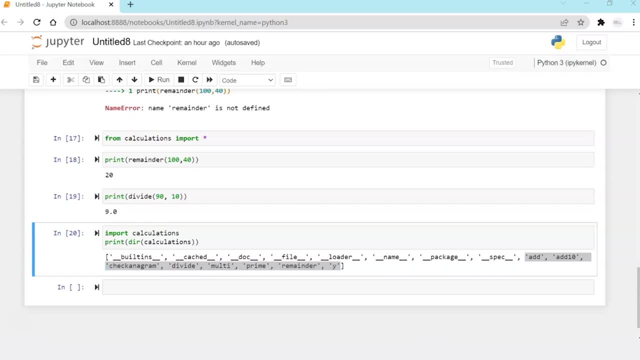 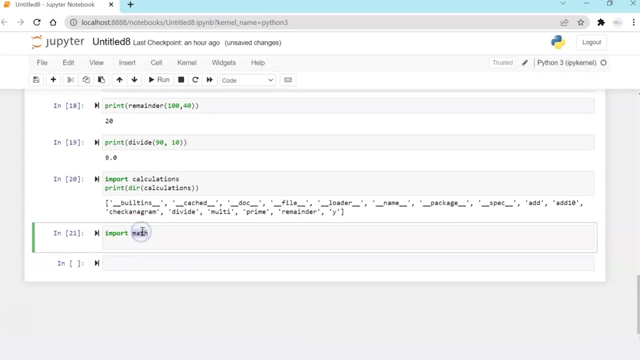 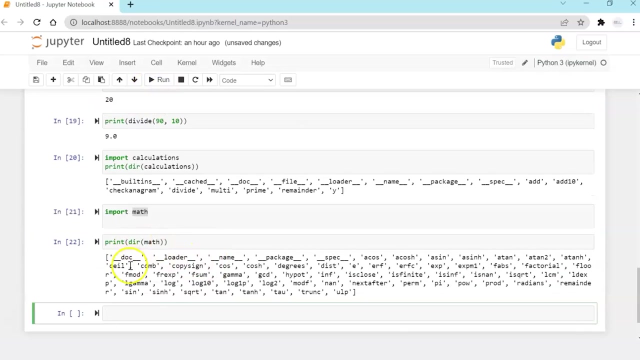 and okay. so now i'm going to show you an example of inbuilt modules. so this import math- math is an inbuilt module of python and i'm going to show you how you can see all the relevant functions within the math module. all these are the math module functions which are available for you. 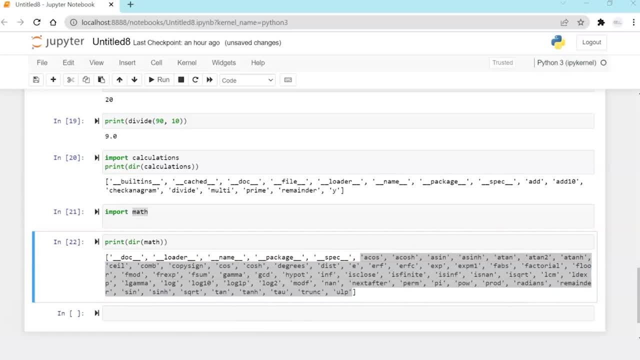 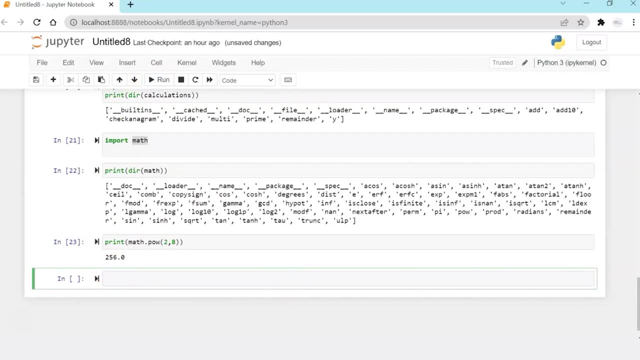 to use. i'm going to show you one or two. so like: print math2 to the plus 0 for the first two factors, 8, and you get the answer 256. print math remainder. so I'm not invoking my module function, I'm invoking the math inbuilt library function remainder and the 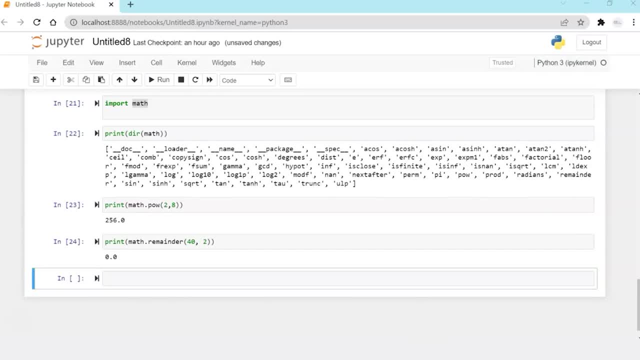 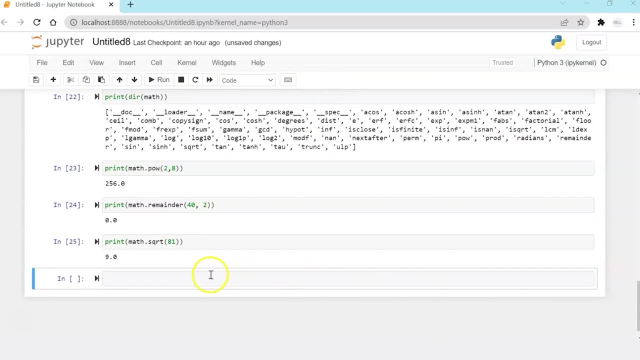 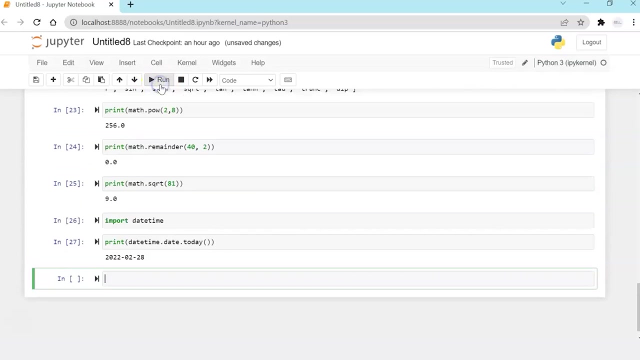 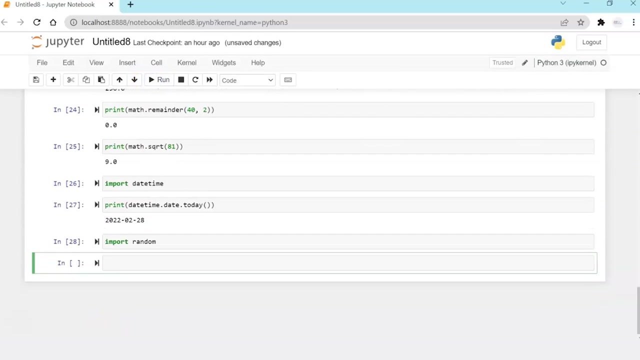 remainder is 0, 40 divided by 2. remainder is 0 and square root of 81: 9. then, very import, another very interesting utilities of date time which you can use and you can print today's date and time. then another utility is random utility and I'm going to create a list, l1, and write a piece of code which will